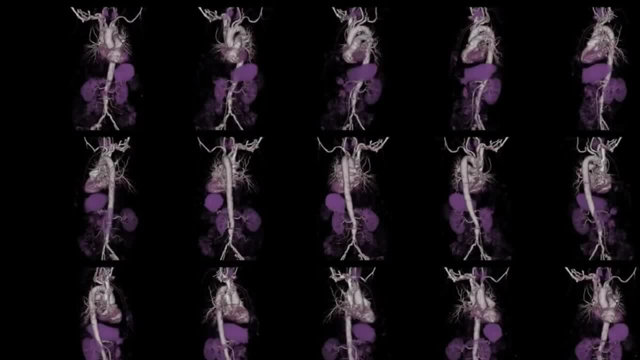 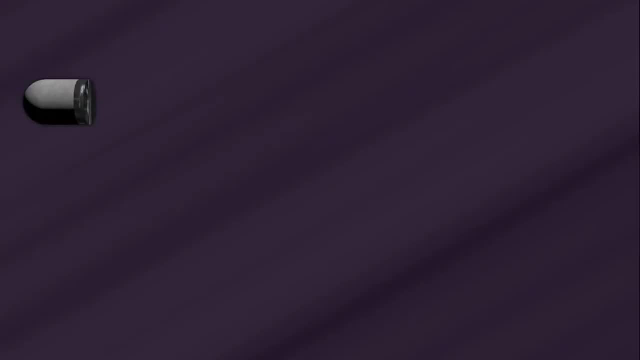 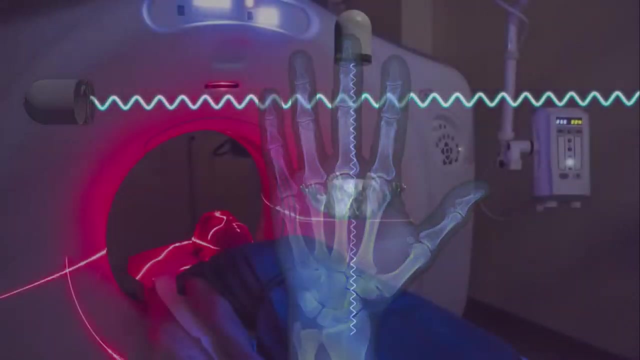 the attenuation coefficient. Using this principle, CT allows the reconstruction of the density of the body by two-dimensional section perpendicular to the axis of the acquisition system. The CT x-ray tube, typically with energy levels between 20 and 150 keV, emits n photons. 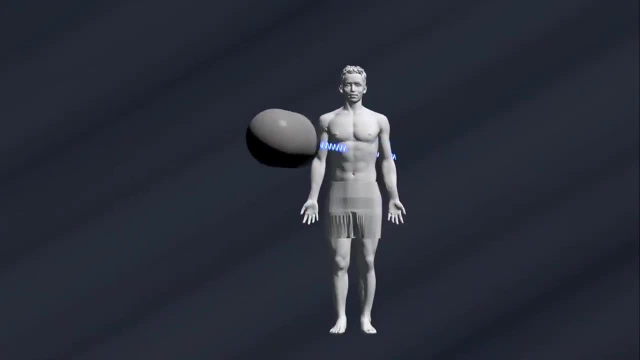 monochromatic per unit of time. The emitted x-rays form a beam which passes through the layer of biological material of thickness. delta x A detector placed at the exit of the sample measures n positive delta n photons. delta n smaller than zero. Attenuation values of the 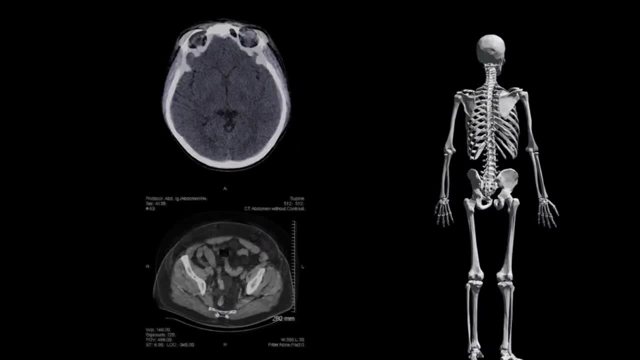 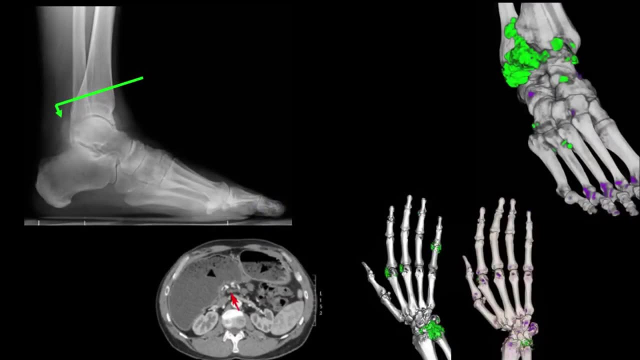 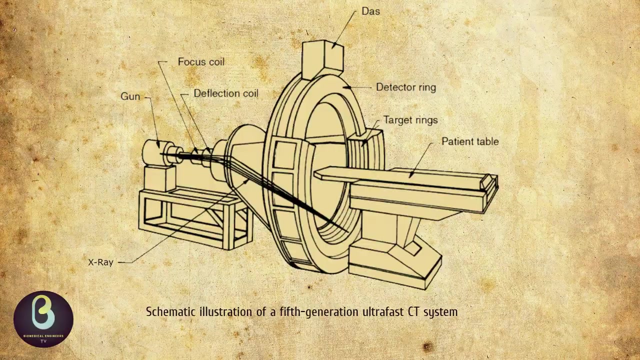 x-ray beam are recorded and data used to build a 3D representation of the scanned object or tissue. There are basically two processes of the absorption: the photoelectric effect and the Compton effect. This phenomenon is represented by a single coefficient. In the particular case of the CT, the emitter of x-rays rotates around the patient. 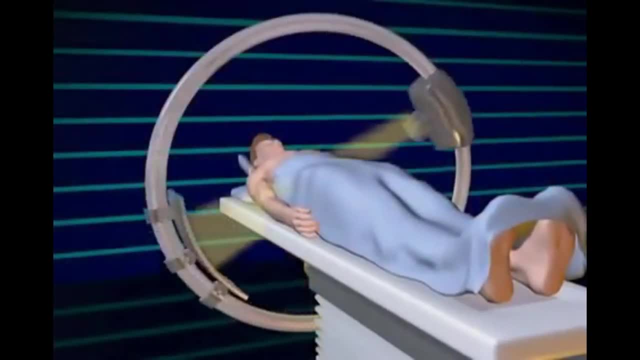 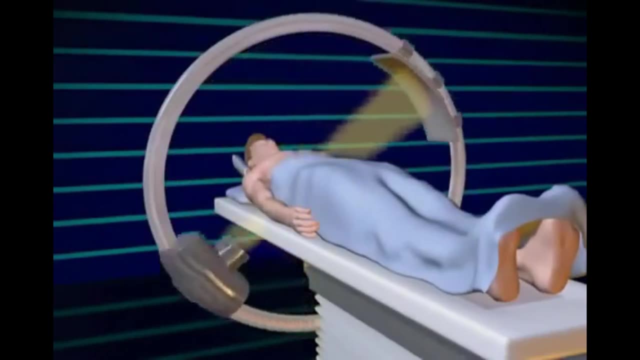 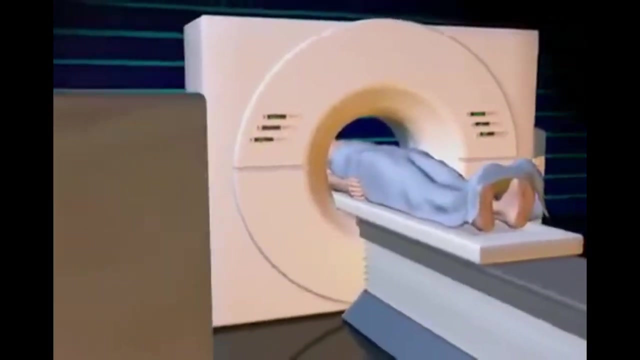 and the detector placed in diametrically opposite sides, pick up the images of a body section. Beam and detector move in synchrony. Unlike x-ray radiography, the detectors of the CT scan are not an image. They measure the transmission of a thin beam- 1-10 mm of x-rays through a full scan of the 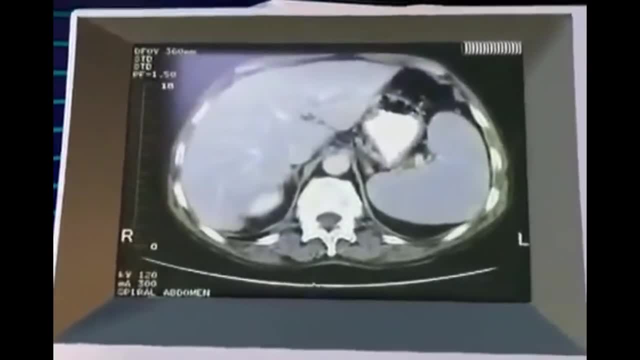 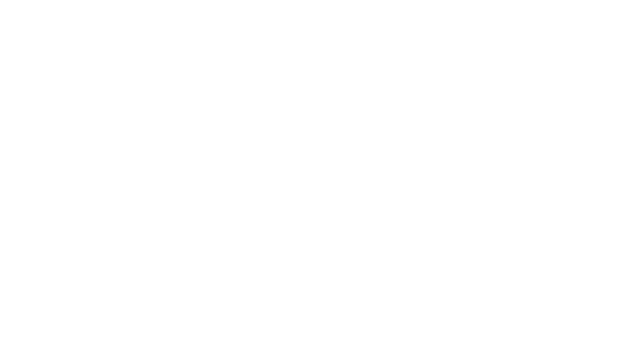 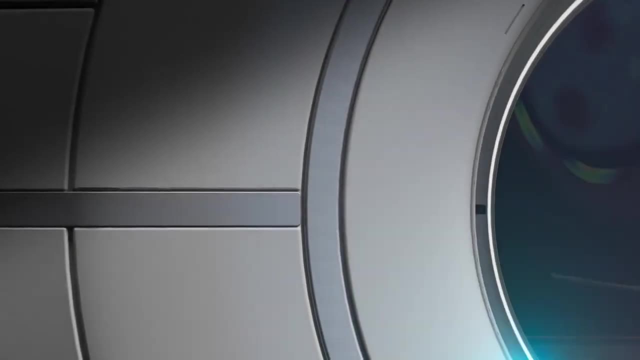 body. The image of that section is taken from different angles and this allows to retrieve the information on the depth in the third dimension. Let's learn about components of CT scanners. CT scanners are composed of three important elements: an x-ray tube, a jantry with a ring. 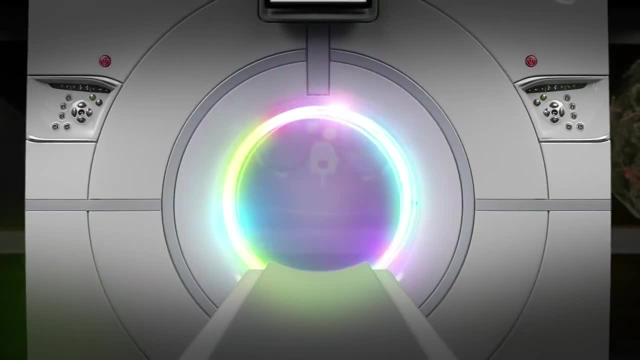 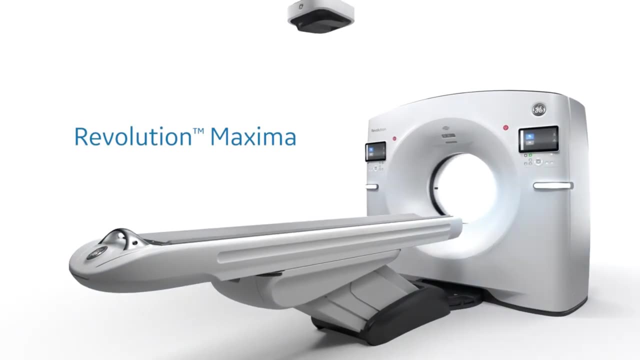 of x-ray sensitive detectors and a computer. First we will look into a jantry. The jantry is the donut-like or ring-shaped part of the CT scanner. It houses many of the components necessary to produce and detect x-rays. These components are mounted on a rotating scan frame. 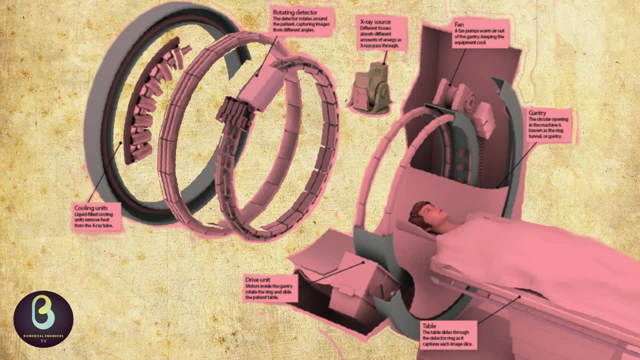 Components of the jantry are mounted onto a rotating scan frame. Jantries vary in total size as well as in the diameter of the opening or aperture. The range size of aperture is typically 70 to 90 cm. The jantry is designed to be tilted either forward or backward as needed to accommodate. 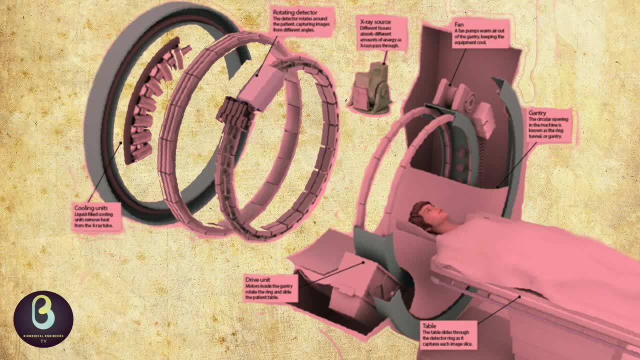 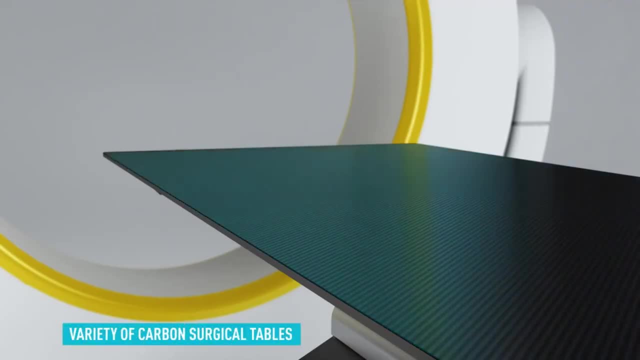 a variety of patients and patients at the same time. A jantry is used to measure the size of an and examination protocols. The degree to which the Jantry can be tilted varies among systems, but more or less 15 degrees to 30 degrees, as usual. 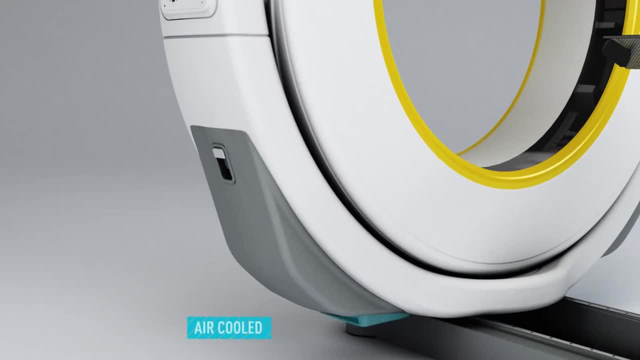 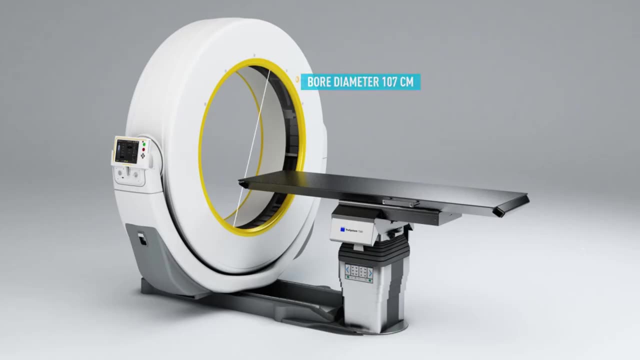 The Jantry also includes a laser light that is used to position the patient within the scanner. Control panels located on either side of the Jantry opening allow the radiologic technologist to control the alignment lights, Jantry tilt and movement of the table. 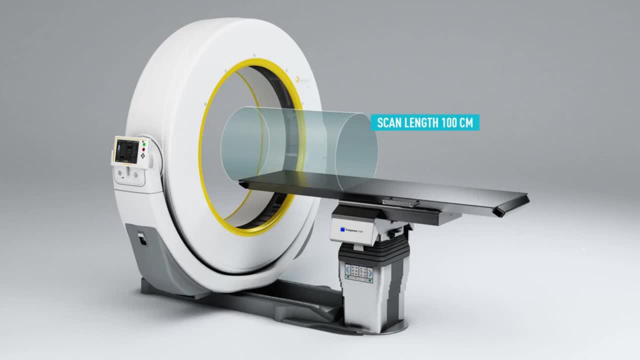 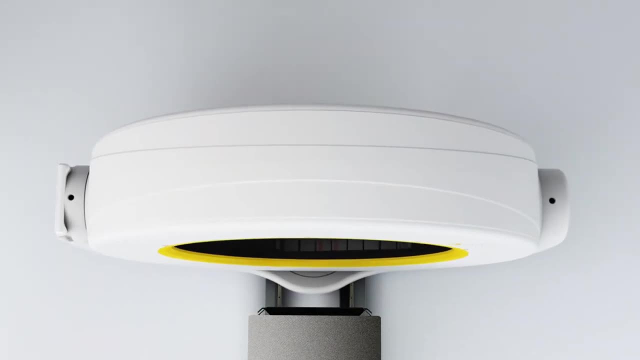 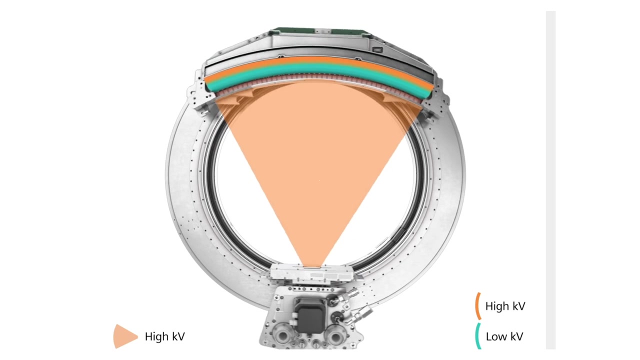 In most scanners these functions may also be controlled via the operator's console. A microphone is installed in the Jantry to allow communication between the patient and the radiologic technologist throughout the scanning procedure. The second component is slip rings. Old model design CT scanners used recoiling system cables. 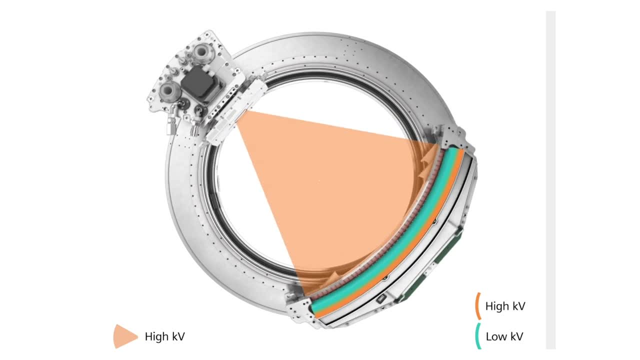 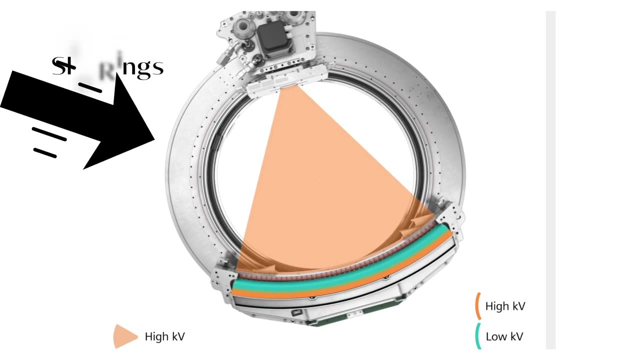 to rotate the Jantry frame. This design limited the scan method to the step and shoot move and considerably limited the Jantry rotation times. Newer systems use electromechanical devices called slip rings. Slip rings use a brush-like apparatus to provide continuous electrical power. 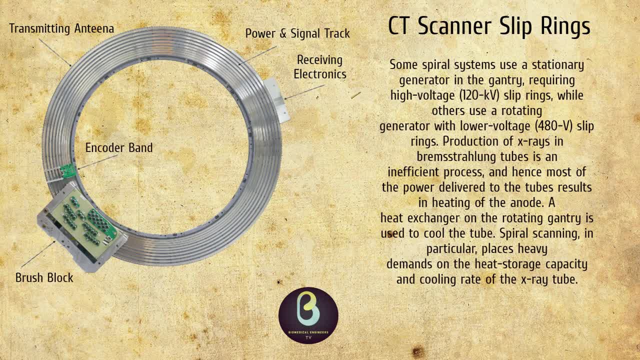 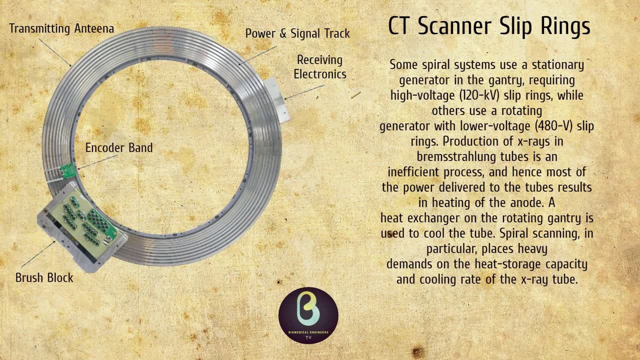 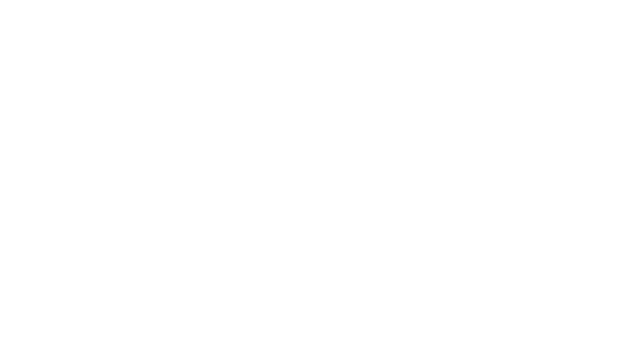 and electronic communication across a rotating surface. They permit the Jantry frame to rotate continuously, eliminating the need to straighten twisted system cables. Slip rings allow the Jantry frame to rotate continuously, making helical scan modes possible. The third component is the generator. 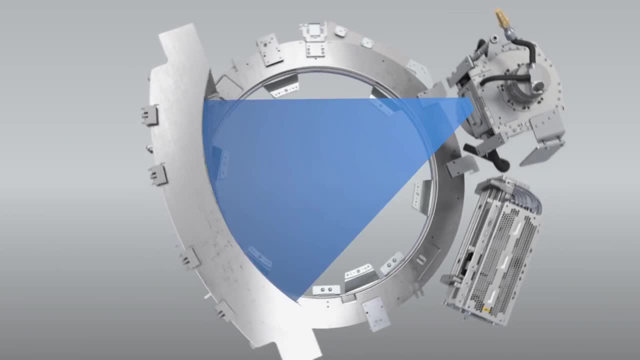 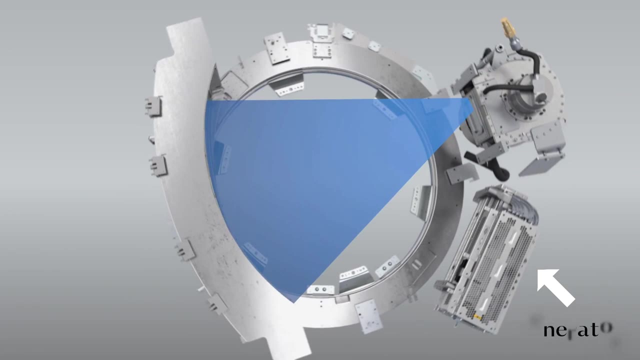 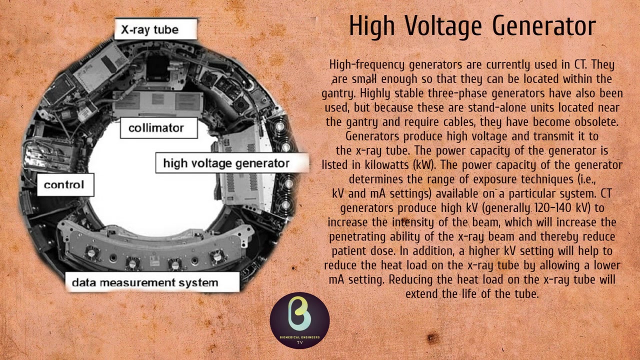 High frequency generator is usually used in CT scanners. The generators are designed to be small enough so that they can be located within the Jantry. Highly stable three-phase generators have also been used, but because these are standalone units near the Jantry and require cables, they have become obsolete. 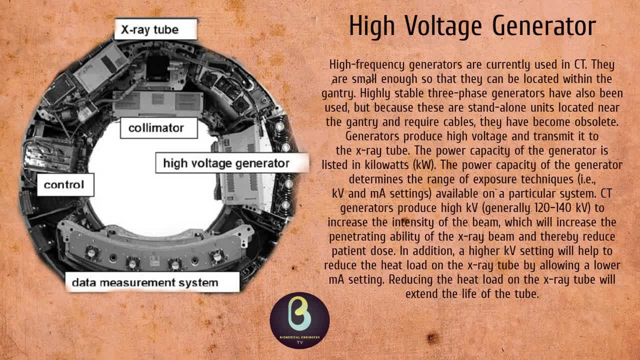 Generators produce high voltage and transmit it to the x-ray tube. The power capacity of the generator is listed in kilowatts. The power capacity of the generator determines the range of exposure techniques like kilovolts and MA settings available on a particular system. 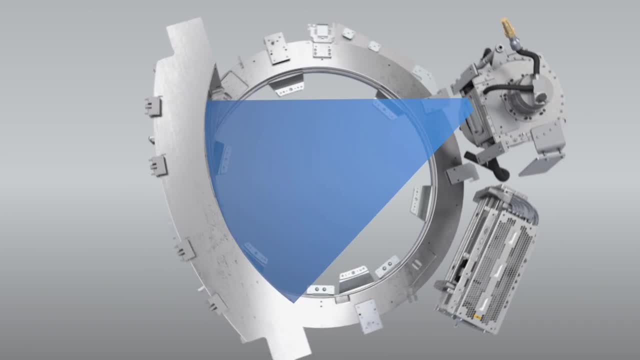 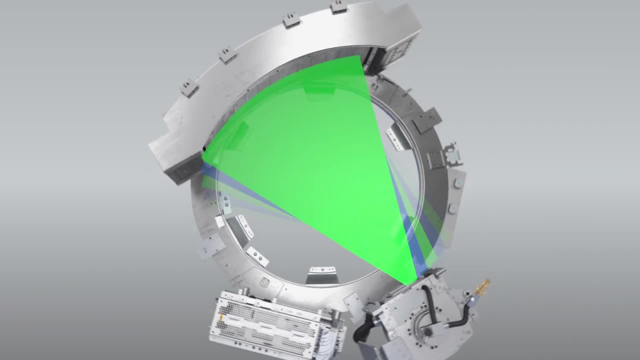 CT generators produce high kilovolts, generally 120 to 140 kilovolts, which is the maximum power generated by the generator To increase the intensity of the beam and thereby reduce patient dose. In addition, a higher kilovolt setting. 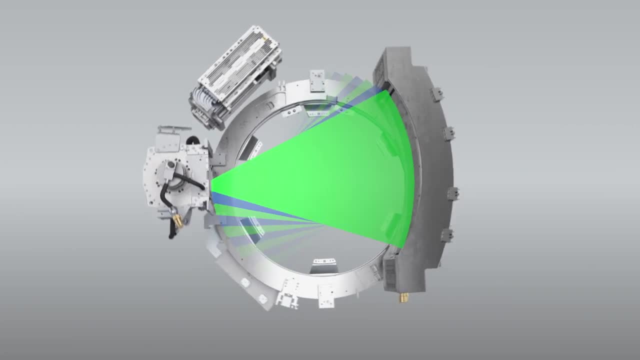 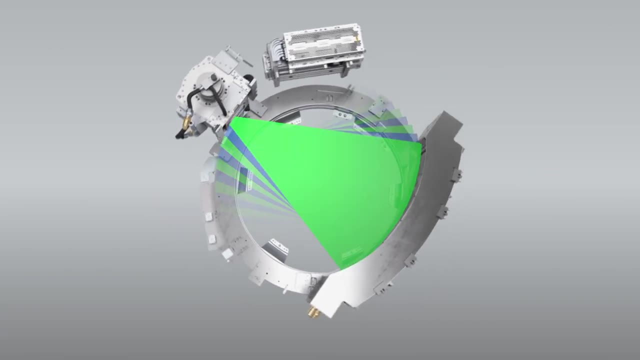 will help to reduce the heat load on the x-ray tube by allowing a lower MA setting, and reducing the heat load on the x-ray tube will extend the life of the tube. The fourth component is the cooling system. Cooling mechanisms are included in the Jantry. 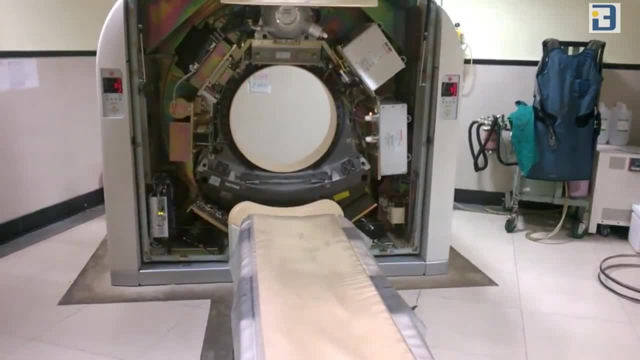 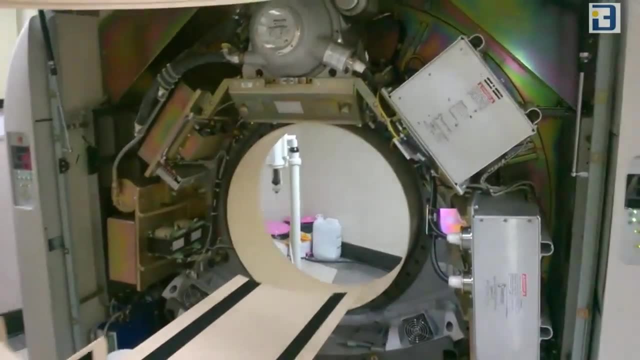 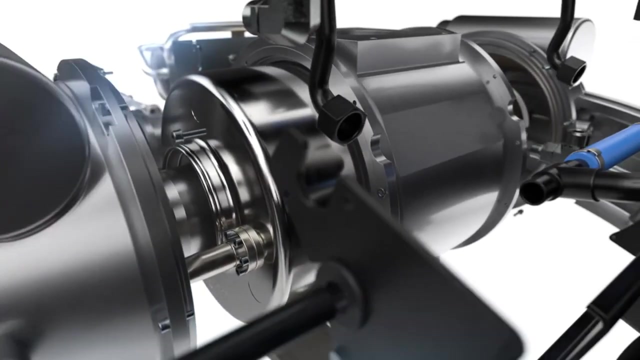 They can take many different forms, such as blowers, filters or devices that perform oil-to-air heat exchange. Cooling mechanisms are important because many components can be affected by temperature fluctuations. The fifth component is the CT x-ray tube. X-ray tubes produce the x-ray photos. 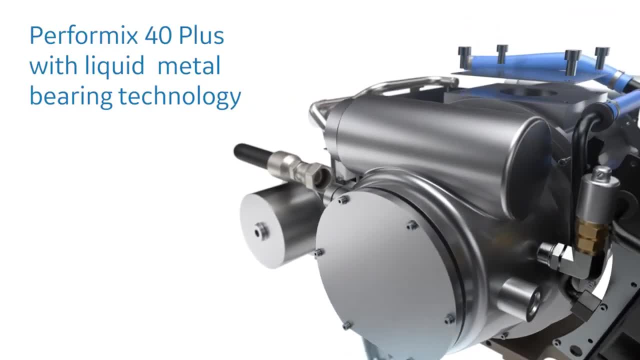 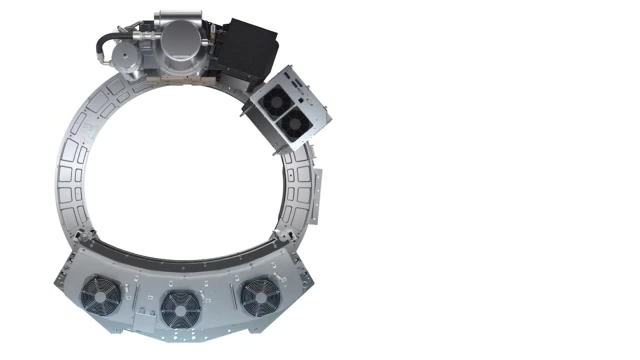 that create the CT image. Their design is a modification of a standard rotating anode tube, such as the type used in angiography. Tungsten, with an atomic number of 74, is often used for the anode target material because it produces a higher intensity x-ray beam. 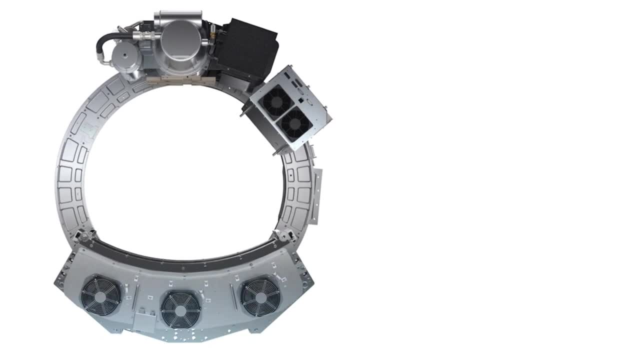 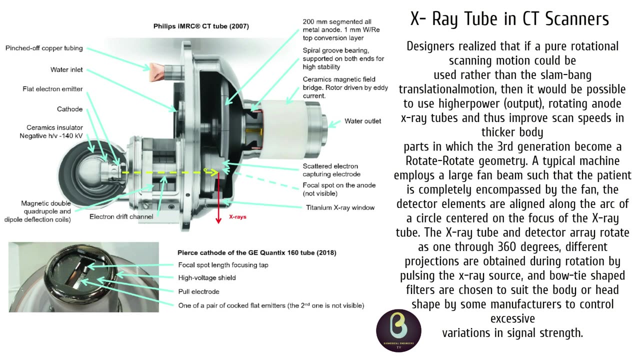 This is because the intensity of x-ray production is approximately proportional to the atomic number of the target material. CT scan tubes often contain more than one size of a focal spot. 0.5 and 1 mm are the common size of a focal spot. 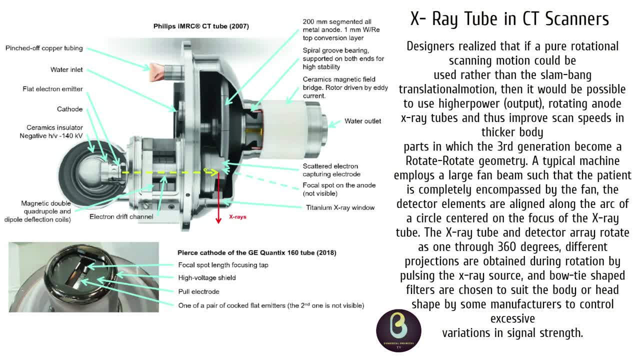 Just as in standard x-ray tubes, because of reduced penumbra, small focal spot and computed tomography tubes produce sharper images, like better spatial resolution, but because they concentrate heat on the smaller area of the anode, they cannot tolerate as much of the heat. 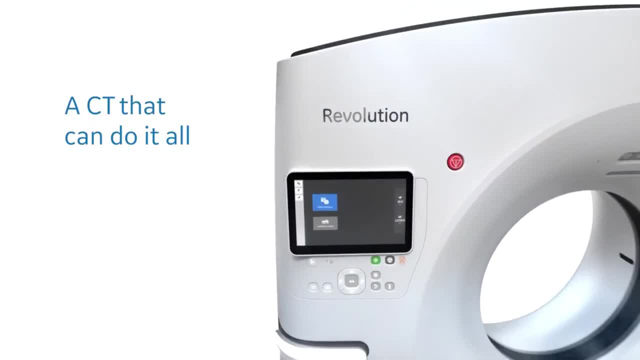 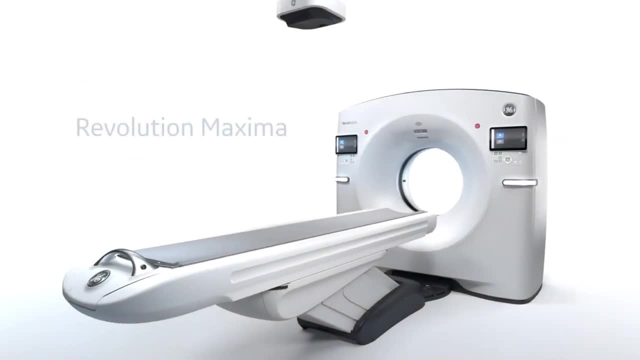 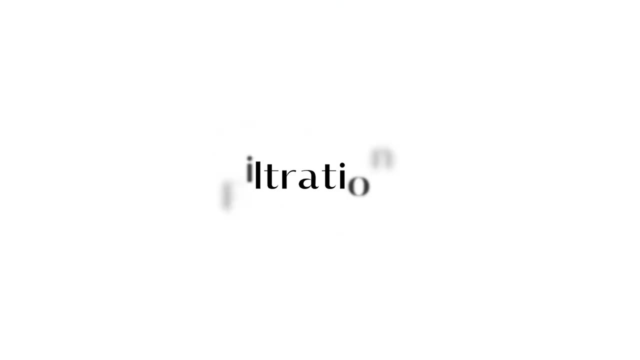 A very large amount of stress is placed on the CT scan tube. Scanning protocols often require multiple lung exposures performed on numerous patients per day. A CT scan tube must be designed to handle such stress. The sixth component is filtration. Compensating filters are used to shape the x-ray beam. 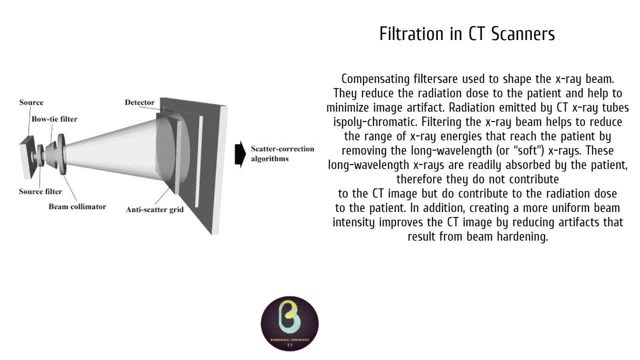 They reduce the radiation dose to the patient and help to minimize image artifact. As our teachers taught us that radiation emitted by a CT scan x-ray tube is polychromatic, Filtering the x-ray beam helps to reduce the range of x-ray energies that reach the patient. 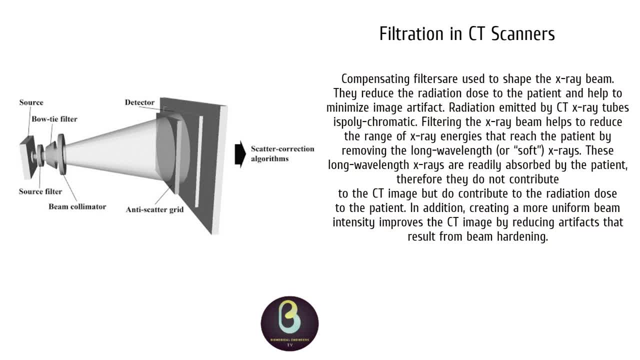 by removing the long wavelength or soft x-rays. These long wavelength x-rays are readily absorbed by the patient. Therefore, they do not contribute to the CT image, but do contribute to the radiation dose to the patient, In addition, creating a more uniform beam intensity. 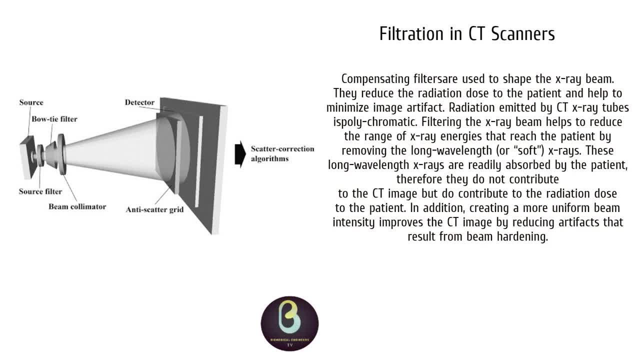 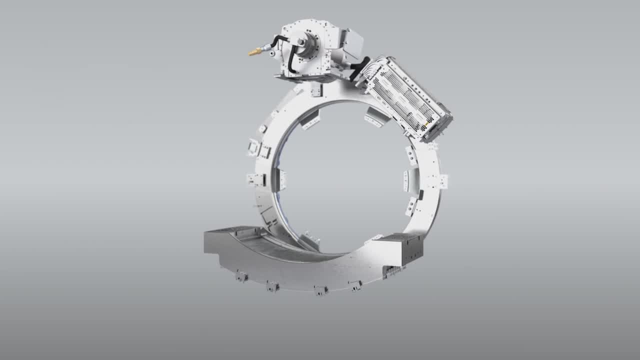 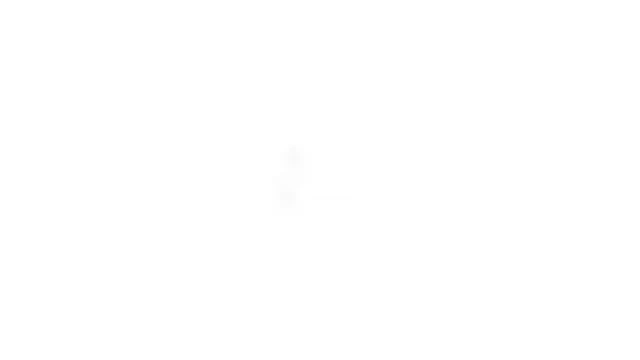 improves the CT image by reducing artifacts that result from beam hardening. Filtering the x-ray beam helps to reduce the radiation dose taken by the patient and it also improves the image quality of the CT scanners. The seventh component is collimators. Collimation restricts the x-ray beam to a specific area. 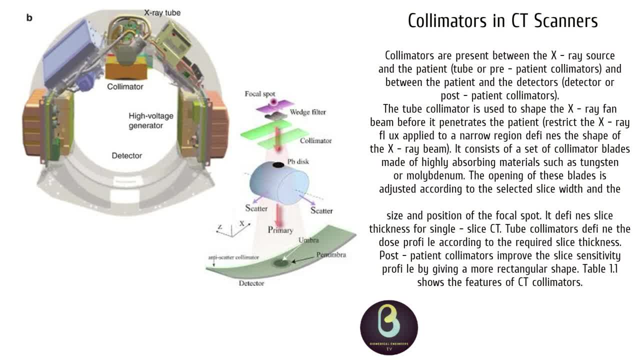 As a result, it helps reduce scatter radiation. This scatter radiation reduces image quality and increases the radiation dose to the patient. Reducing the scatter radiation improves contrast resolution and decreases patient dose. Collimation controls the slice thickness by narrowing or widening the x-ray beam. 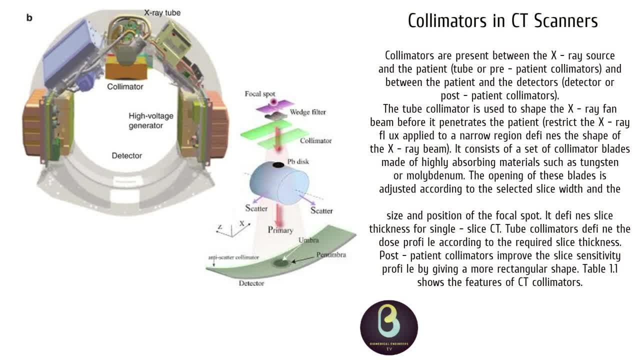 The source collimator is located near the x-ray source and limits the amount of x-ray beam before it passes through the patient. It is sometimes referred to as patient dose and determines how the dose is distributed across the slice thickness. like the dose profile, The source collimation resembles small shutters. 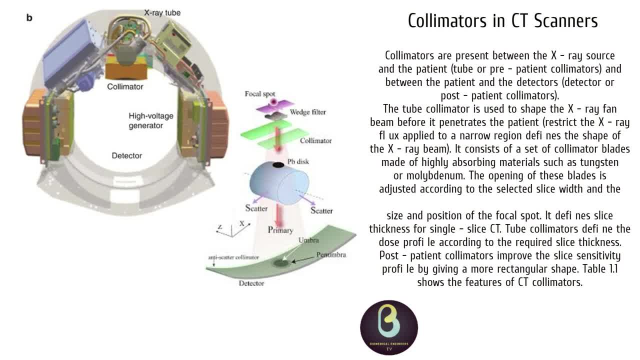 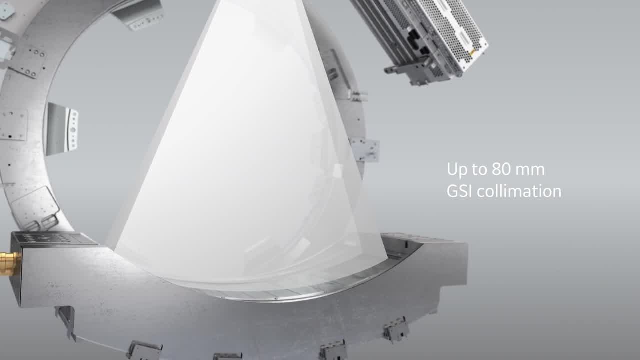 with an opening that adjusts, dependent on the operator's selection of slice thickness. In MD-CT systems, slice thickness is also influenced by the detector element configuration. Scanners vary in the choice of the x-ray beam and the choices of slice thickness available. 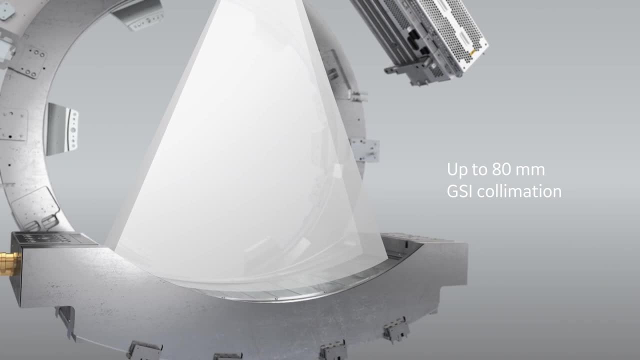 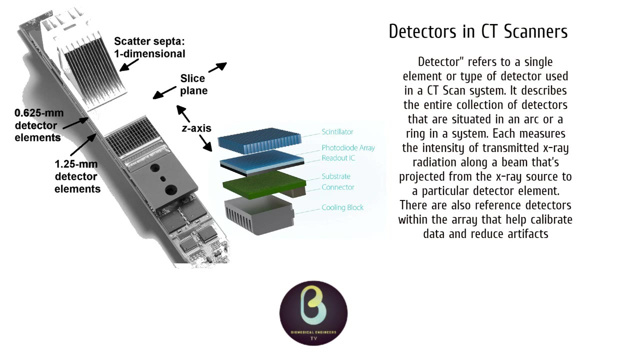 Choices range from 0.5 to 10 millimeters. And the last but not least component are the detectors. The detectors are components of CT scan machines which collect information regarding the degree to which each anatomic structure attenuated the beam. In conventional radiography, we use a film screen system. 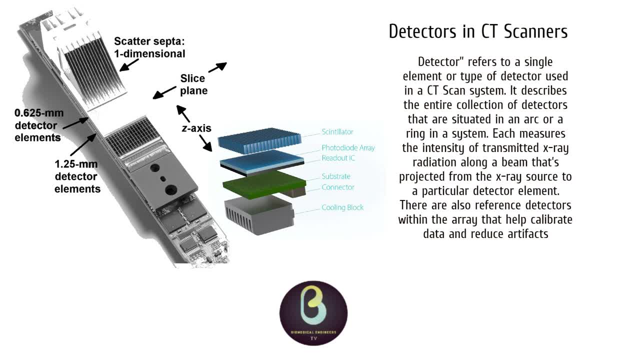 to record the attenuated information. In CT, we use detectors to collect the information. The term detector refers to a single element or a single type of detector used in a CT system. The term detector array is used to describe the entire collection of detectors. 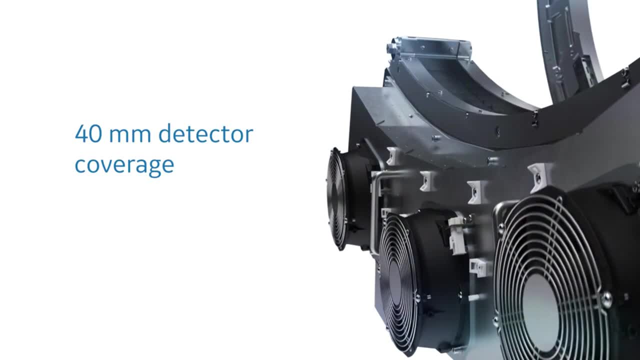 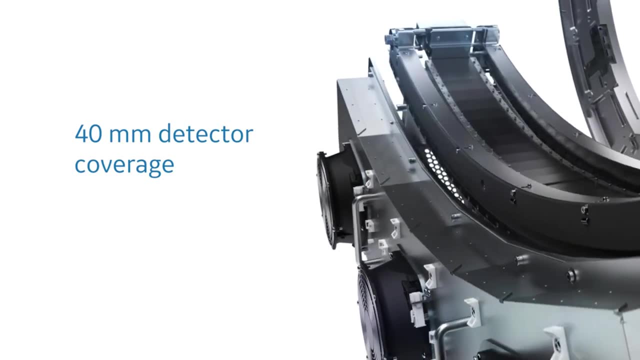 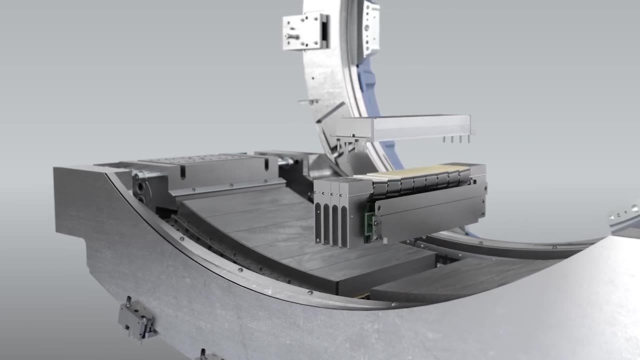 included in a CT scan system. Specifically, the detector array compromises detector elements situated in an arc or a ring, each of which measures the intensity of transmitted x-ray radiation along a beam projected from the x-ray source to that particular detector element. Also included in the array are elements referred to: 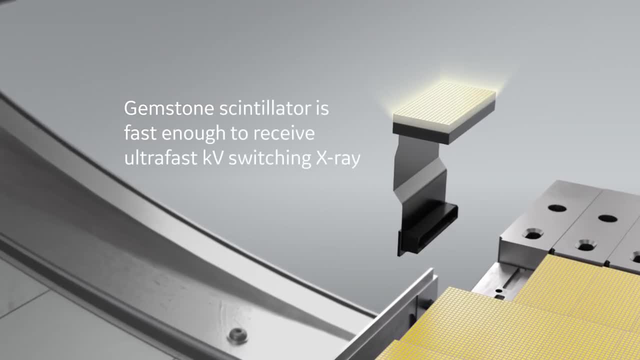 as reference detectors that help calculate the intensity of the beam. Also included in the array are elements referred to as reference detectors that help calculate the intensity of the beam. Also included in the array are elements referred to as reference detectors that help calculate the intensity of the beam.